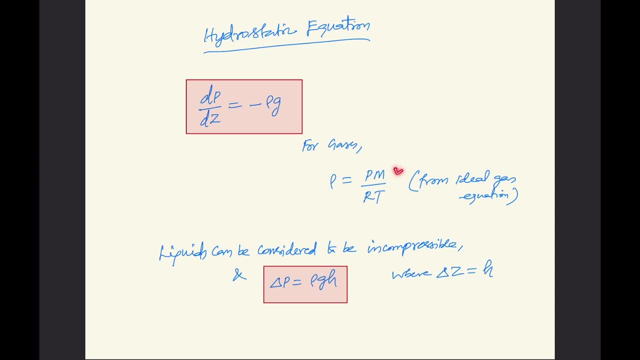 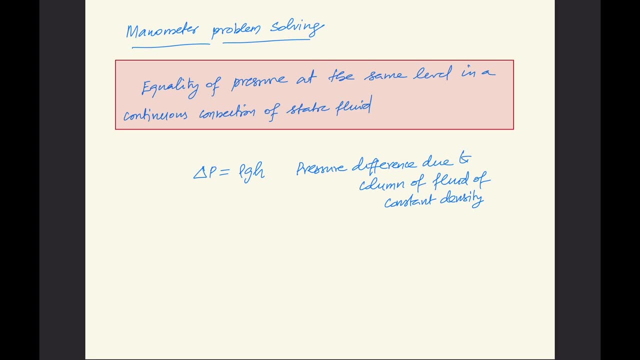 ideal gas equation simply given by rho, equal to pm by rt, And one of the essential use of this hydrostatic equation is for manometer problems, wherein which we have this concept. there is equality of pressure at the same level in a continuous connection, of static fluid, For example. we will apply this Say, for example, in this: 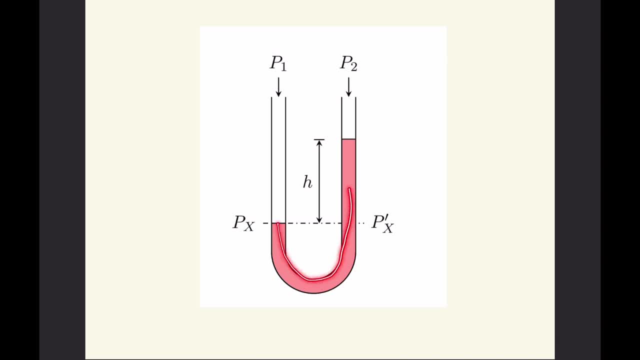 manometer. we have this manometric fluid. Of course it is continuous at this level. We have a continuous connection of manometric fluid at this level. So we can equate pressure at x and x dash. Pressure at x will be based on p1 and pressure at x dash is based on p2, plus this column of fluid. 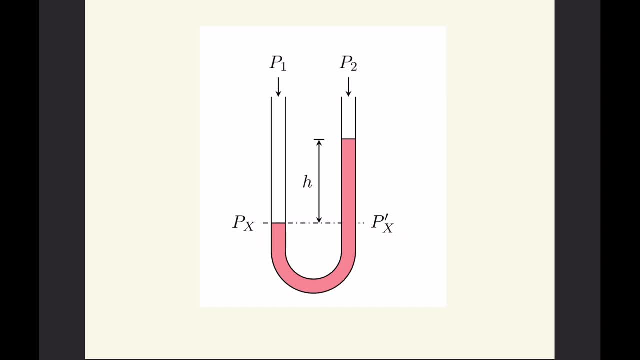 And we can equate this px and px dash and we can get the difference between p1 and p2.. Say, for example, if the manometer is having many fluids, influx also will create the added px of p1 and p2, plus this px into p2, plus this px into 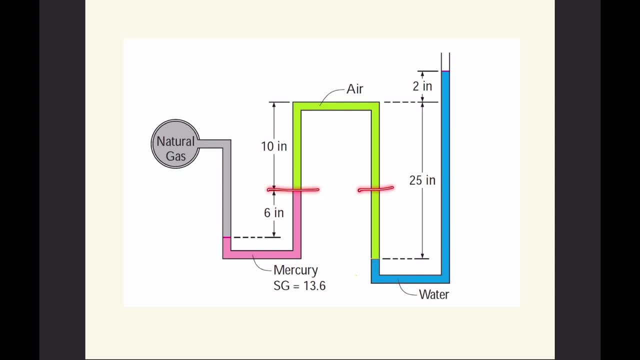 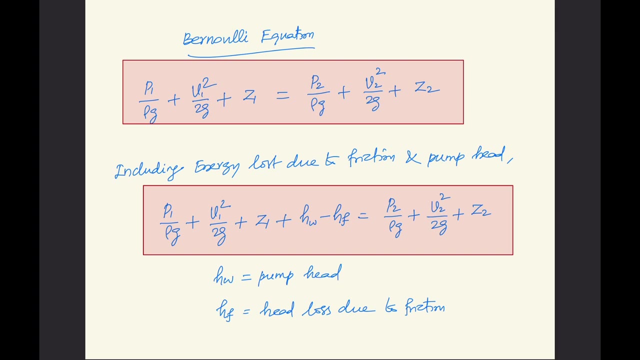 p2 plus this px. So we get that this same result as being effective for all fluids. So for another person, this is minute alter and this gives you quick equation process. Warming of all fluids is final B In this equation. there are a total number of liquid substances like valence as a power. 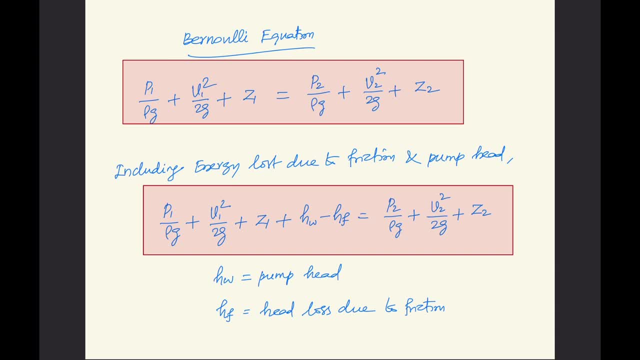 bar and a grasses, larger roles plus the맛. So we can give only p Plan, which is a little strong, So that that gives us a fluid moment of P1 times, so we can evaluate the pressure at this level, whereas we have this continuous connection of water and also at this level, 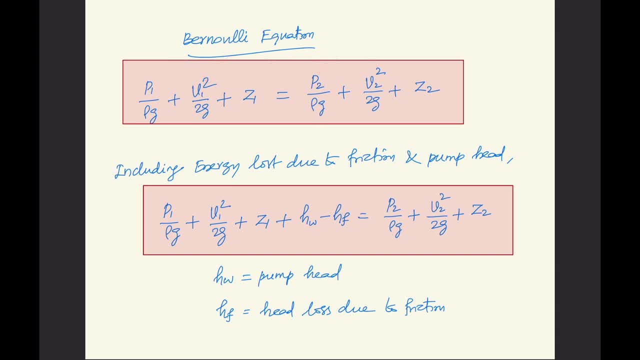 wherein which we have a continuous connection of air, and also, at this level, wherein which we have a continuous connection, of mercury by 2g plus z1, equal to p2 by rho, g plus p2, square by 2g plus z2.. Including the frictional losses and head added by the pump, we can add these two terms there. 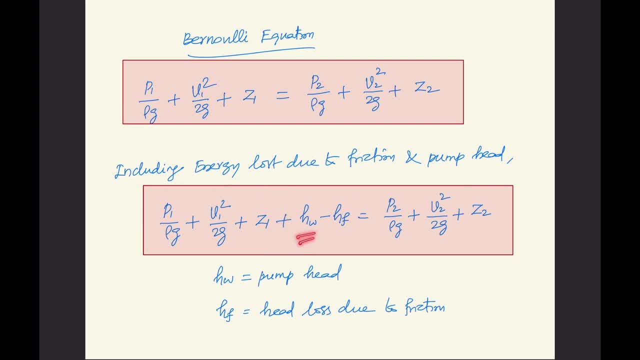 is energy at 1 plus energy added by the pump. of course everything is in terms of head of the flowing fluid minus energy loss due to friction. that is equal to energy at 0.2.. So this hw is the head added by the pump and hw is the head loss due to friction. 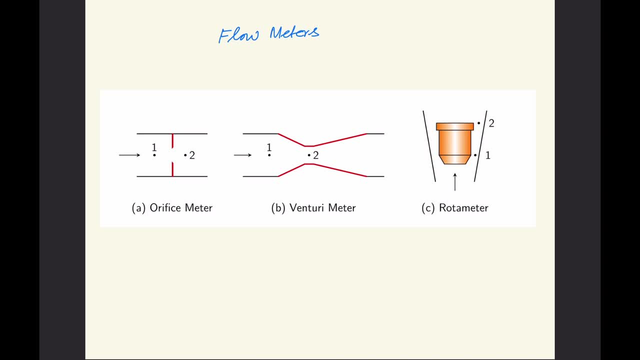 One of the common usage of this Bernoulli equation is for the flow meters getting the equation for velocity at the point of this reduced cross-section, or even in the case of measuring the flow using a rotameter, using the devices. Of course, the most common used devices are RFS meter, Venturi meter and other devices. 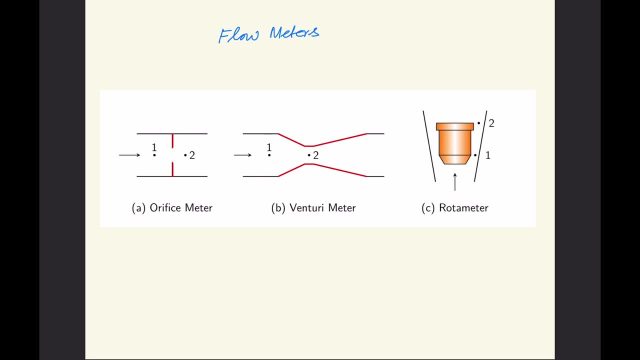 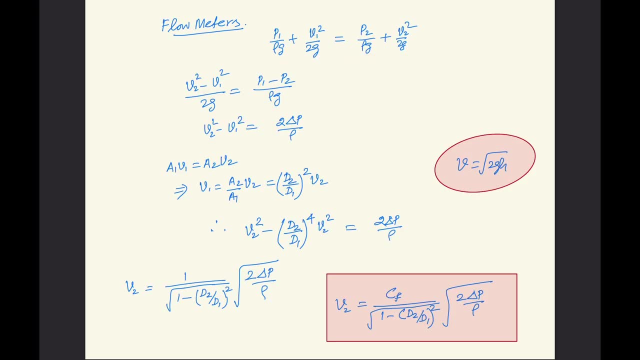 All these flow meters are based on the application of Bernoulli equation. For example, we have this Bernoulli equation: since point 1 and 2 are at the same level, we can subtract them, we can cancel out them, So we have this velocity expression coming out in terms of pressure difference. this 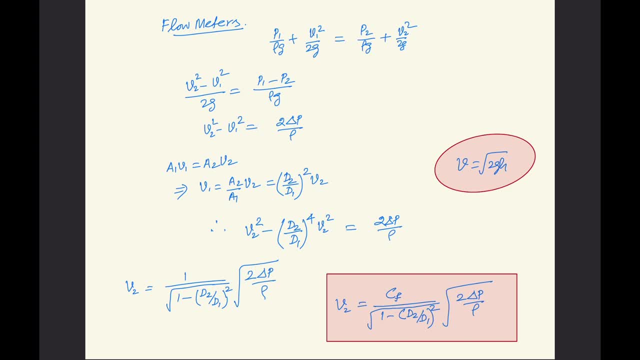 pressure difference is this: delta p refers to p1 minus p2.. So we have this simplest equation here, in which we have these terms: diameter ratio and pressure difference. this is actually. this equation is obtained by assuming no energy loss in the form of friction, whereas including frictional losses- we have the term, we have. 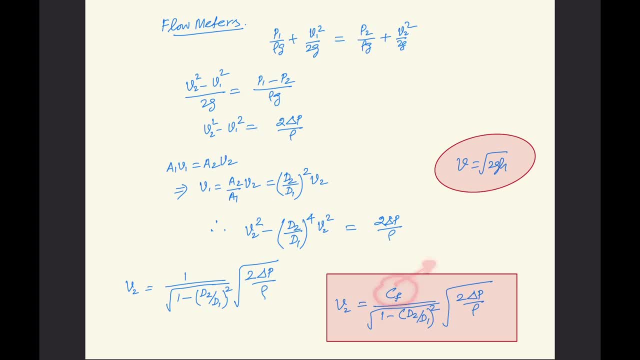 the equation with a term what is called as flow coefficient, Venturi coefficient or RFS coefficient or coefficient of rotameter See. So this equation is common for all these devices, whether it is Venturi meter, RFS meter or rotameter. 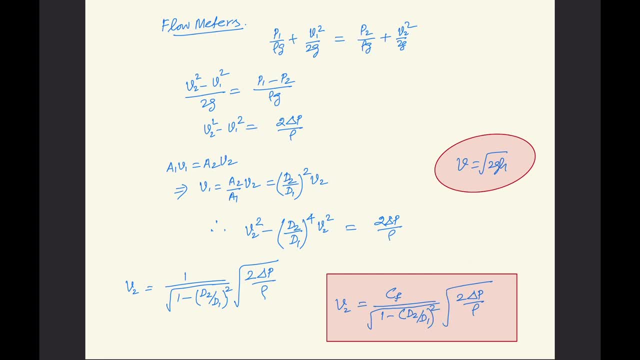 For rotameter, this group is a constant, whereas this is a variable, whereas for Venturi and RFS, this group is remaining constant, whereas this delta p is a variable. Of course, this equation is in simple. we can simply relate this to: v equal to root 2gh. 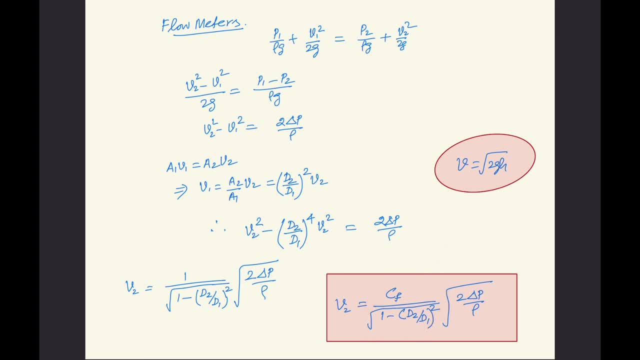 in what way? So this can be simple: constant and this delta p by rho is nothing but rho gh or it's delta p equal to rho gh, so from which we have v equal to v is equal to root 2 gh. 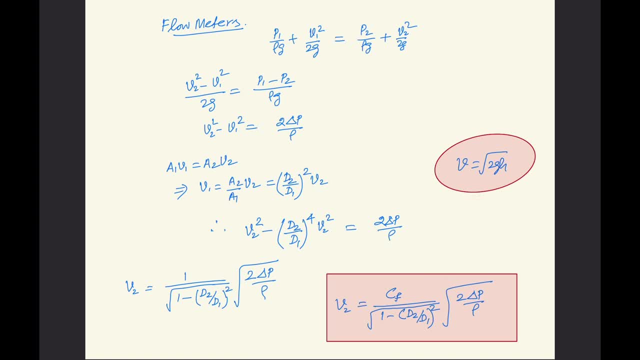 or if we can easily obtain from this, we can easily say this: v is also equal to root 2, gh. Of course, this flow coefficient is simply taken as one here, and also the ratio area ratio is. this term is simply taken as one and we can get the relation between wall shear stress and 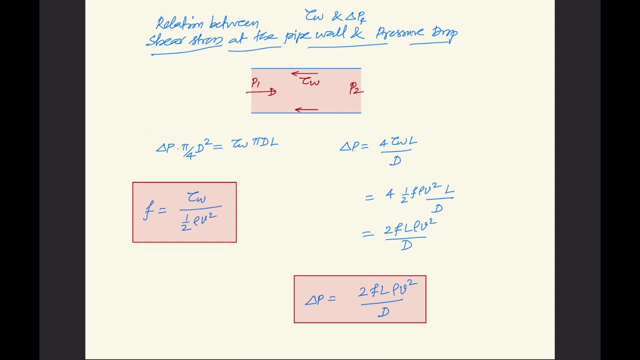 this frictional pressure drop by making this balance. this pressure difference is pressure difference multiplied by the area over which it is acting. that is, the pressure force is acting on the entire circular cross section, whereas this wall shear stress is acting on the pipe surface area, which is pi d. L is the area over which wall shear stress is. 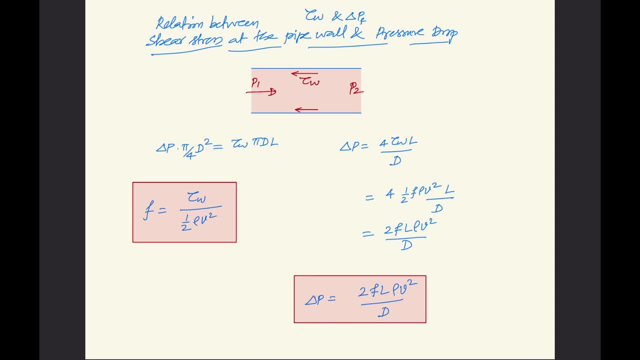 acting, whereas the delta P is acting over this pipe cross section, flow cross section. this is flow cross section. this is what is called as a wetted area of the pipe. so from these, by equating this, we have this relation: delta P equal to 4 tau dash. 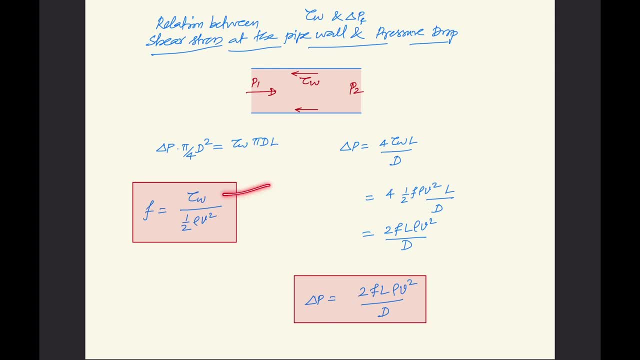 W, L by D, and using the definition of F, which is F equal to tau, W by half rho V square, we can get this nice equation: delta P equal to 2 F, L, rho V square by D. Again to remind you this F is actually fanning friction factor. In civil and mechanical engineering they use the another. 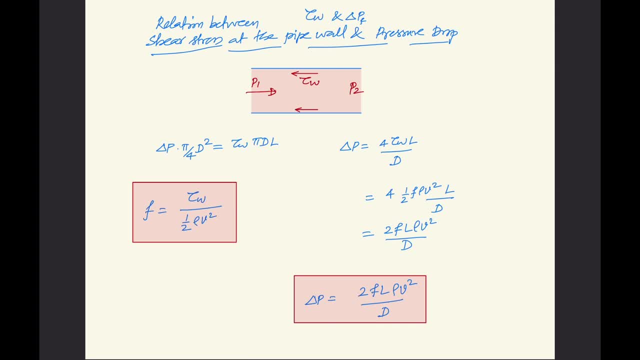 friction factor, what is called as Darcy or Blasius friction factor. So otherwise this equation, instead of 2 appearing in the numerator in the books of civil and mechanical they used to have this 2 in the denominator, where in which they, in place of F, they use F, D, Otherwise F, whatever we 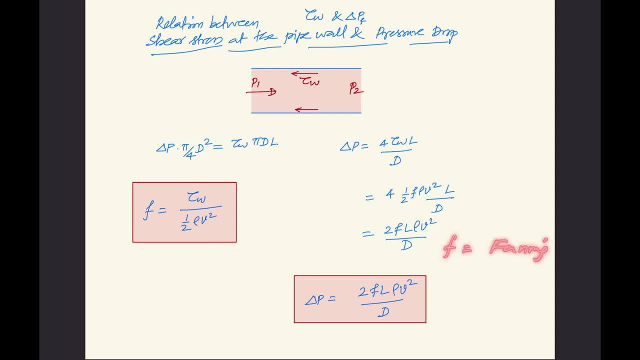 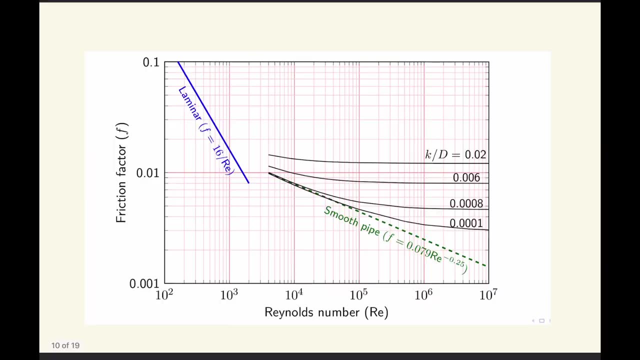 use here is fanning friction factor. Again delta P equal to 2 F L rho V square by D. Yeah, this is a friction factor. Reynolds number relationship F equal to 16 by Reynolds number in the laminar. Otherwise F is having for a smooth pipe. the most common used equation is 0.079 R e to the power. 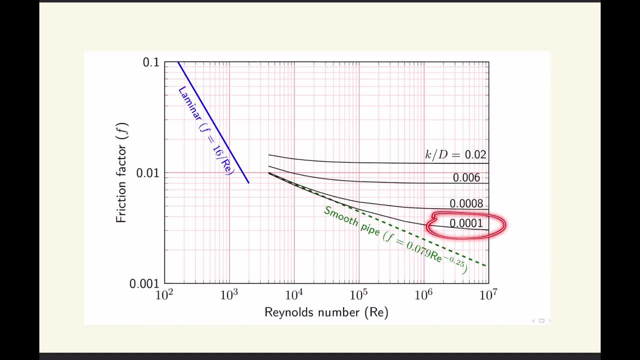 minus 0.25.. Otherwise, for rougher pipe it is a function of roughness. with increase in roughness, F also increases. Almost after this 10 power 6. we can say like this, F is remaining constant. Of course, for smooth pipe it is keep on decreasing. 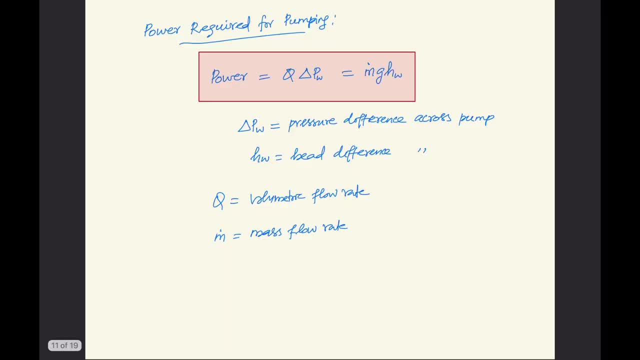 Functional relationship is also needed And for estimating the power loss, sorry, estimating the energy required for pumping delta P equal to molymetric flow rate into pressure difference across the pump. Otherwise, we can also write in terms of mass flow rate as m, g, h, m dot g. 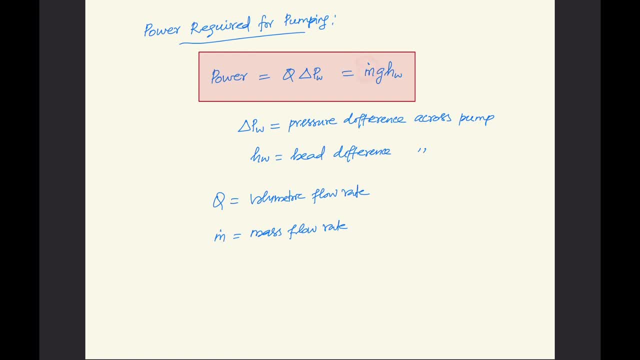 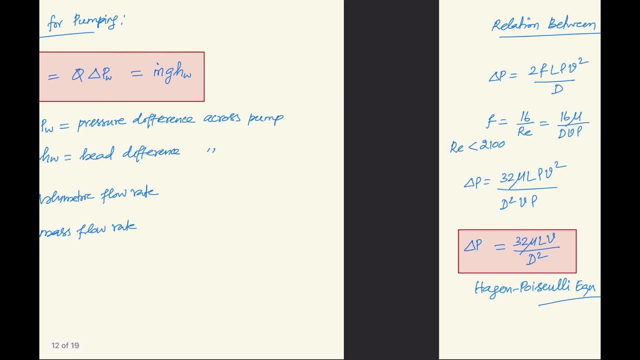 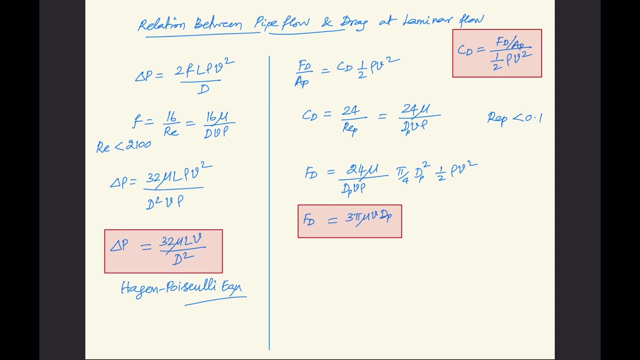 h, m, g, h is energy, m dot is mass flow rate into g, h, w, So otherwise m dot is mass flow rate, So energy by time. we have this power. Okay, Thank you. And we can relate this pressure drop due to pipe with this drag force per unit area in: 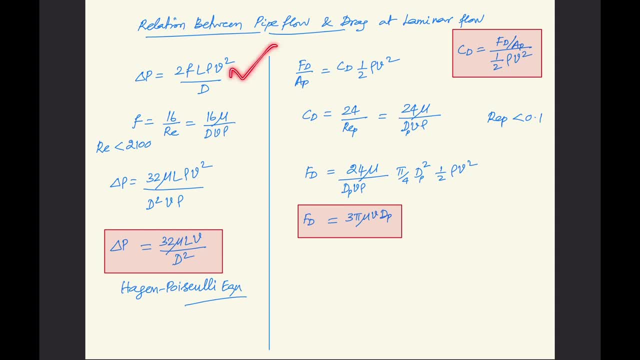 the case of drag flow: Flow around a solid. This is flow through pipe and this is flow around a solid. This delta P is force, or is this also force per unit area? That's why here also we have this drag force per unit area. In place of F, we have C d here, So this: 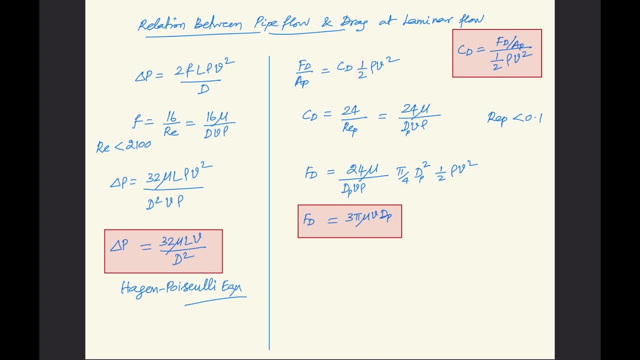 is here. Here we have half rho v square. Instead of half rho v square, we have actually 2 rho v square. Okay, In seeing this connection, this F equal to 16 by Reynolds number in laminar flow and F equal to 24 by Reynolds number particle for what is called as creeping flow. 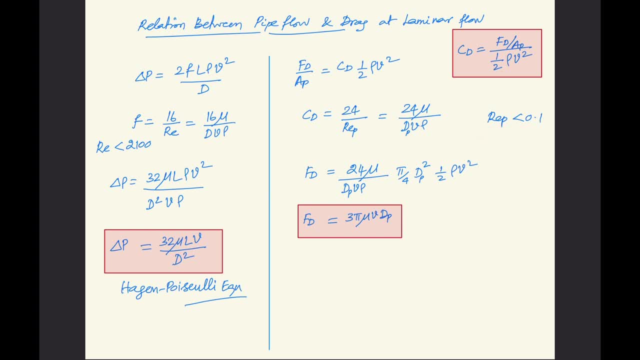 which is valued for Re particle lesser than 0.1.. So what is Re particle which is D p? rho, D p? v? rho by mu? So, except particle particular which is constant? we have R? e, So we have D? p? rho by mu, So we have 0.8 V? rho by mu, So D plus is equal to 0.4.. So d plus is equal. to 0.8 V rho by mu. So d plus is equal to 0.8 V rho by mu. So we have F equal to 10 to the greater than 0.8 V rho by mu. So this is the normal umas if we consider the temperature from. 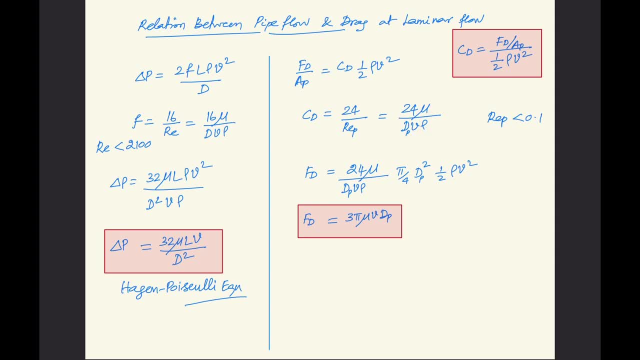 the particle diameter. the other things are fluid properties from which, for laminar flow situation, we will be getting FD equal to 3 pi, mu, V dP. This is the equation, what is called as, which is also called as Stokes law, and we, for the same case, for the pipe flow, we 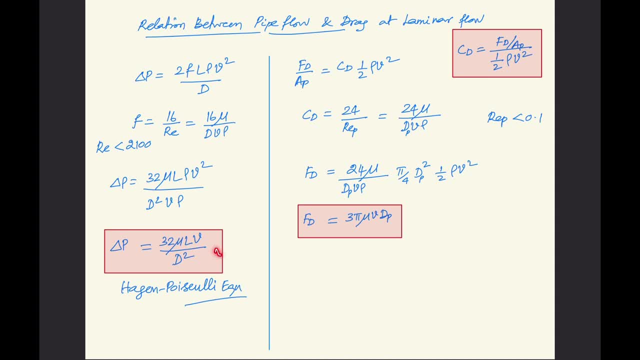 have delta P equal to 32 mu L V by d square. This is what is also called as Hagen Beisele equation. So of course both the equation have the same functional dependency with velocity and viscosity. So FD is proportional to viscosity and velocity. here also we have delta P is. 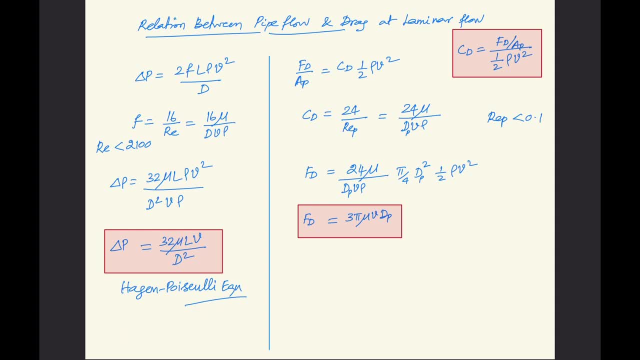 proportional to velocity. viscosity and velocity, Of course, both either flow through pipe or flow around solid. both have the same kind of dependency with velocity and viscosity And, of course, the same relation. what is this? we have a plot of drag coefficient with such Reynolds number for lower Reynolds number. 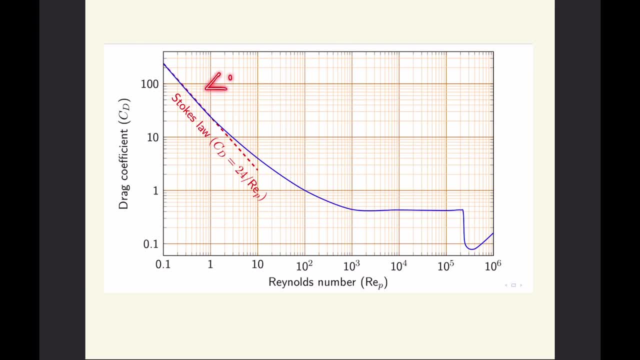 less than actually 1, or better to take it as less than 0.1.. We have a linear relationship between not actually linear linear in the logarithmic scale: CD is equal to 24 by Reynolds number, particle for Rep less than 0.1, even up to 0.1. also, this dashed line, dashed red. 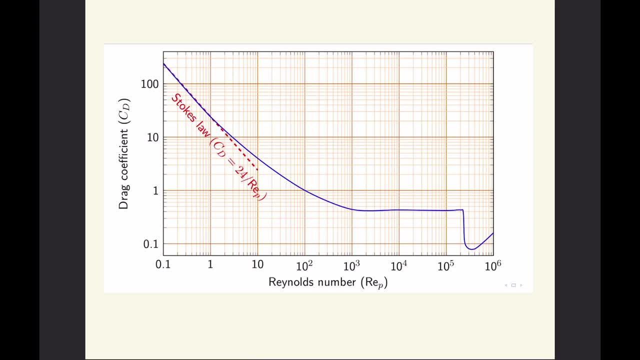 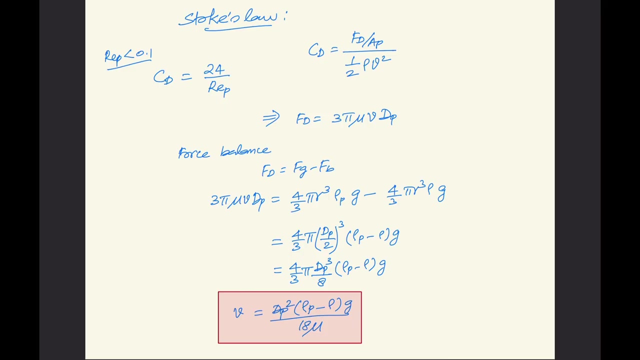 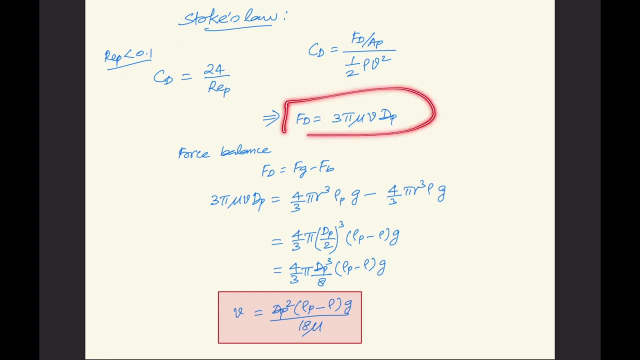 we have. What we have is this: UZ what we can do. thisёт require: if theệt value is equal to Well, if the철 value is equal to Re, we have to take the force BET. So this is what we. 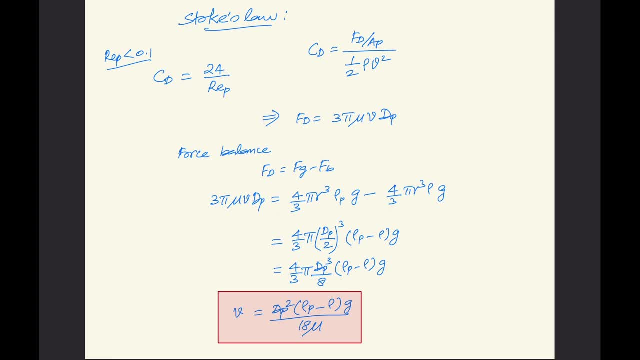 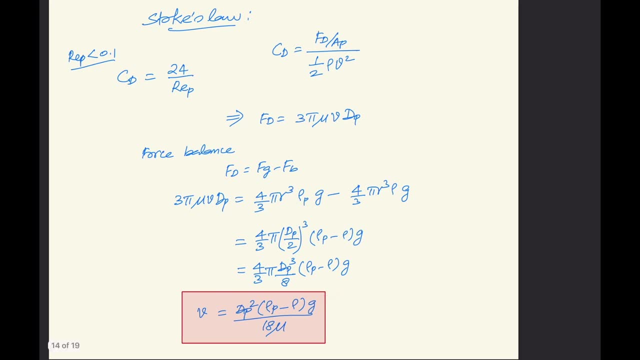 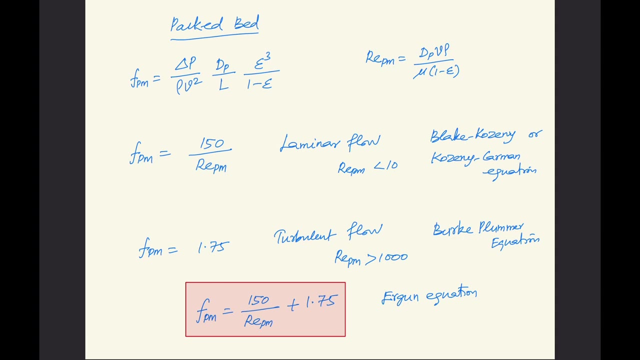 have this total force equal to, we have to take the force epsilon and then to get the range which is dp square into rho, p minus rho into g, by 18 mu and coming to the flow through bed of solid, what is called as a packet bed. we have these definitions of f: porous, medium and re porous. 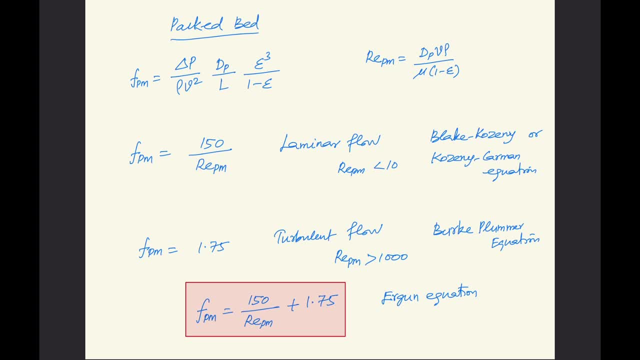 medium. f porous medium is defined as delta p by rho v square. dp by l into epsilon cube. by 1 minus epsilon, epsilon is void h or porosity. you can of course delta p by rho v square in. this is easily understandable. delta p by rho v square is a dimensionless quantity. dp by l is a dimensionless. 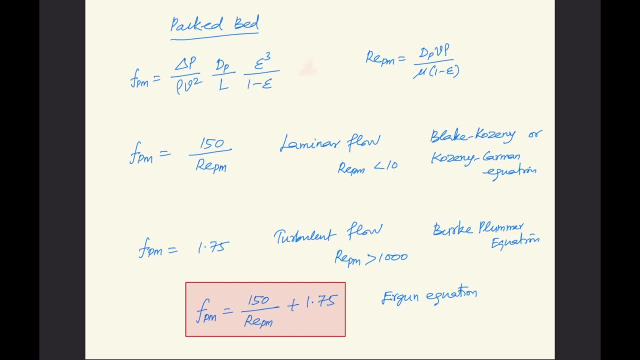 quantity, and e is already. epsilon is already a dimensionless quantity. of course, here delta p by l should come. that's why we have this delta p and dp by l. don't write it as l by dp. delta p by l is needed, so that's why this delta p by rho v square multiplied by dp. 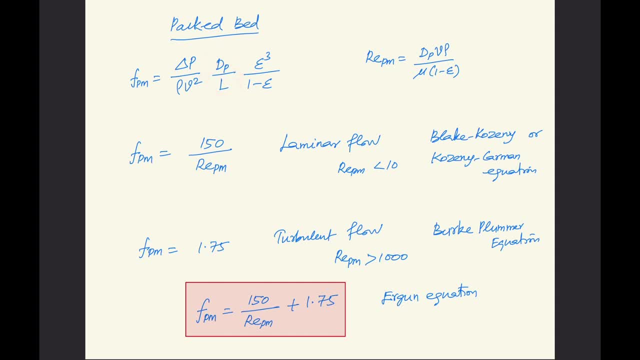 by l. that is, if you expand this, you'll be having as delta p by l. directly. okay, which is near what is called as pressure gradient, and repm is given as dv rho by mu. of course d is dp, what is called as particle diameter, dv rho by mu by 1 minus epsilon. this 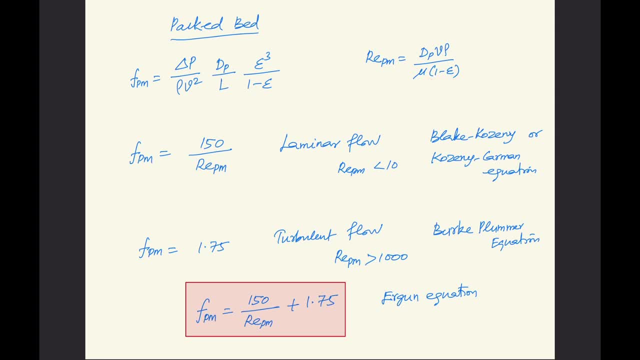 epsilon, as i already said, void h or porosity. okay, for the laminar flow we have, this relation: f- pm is equal to 150 by repm. and what is that? for flow through pipeline, f is equal to 16 by re. and for the case of flow around a solid, what is called as a creeping flow drag, 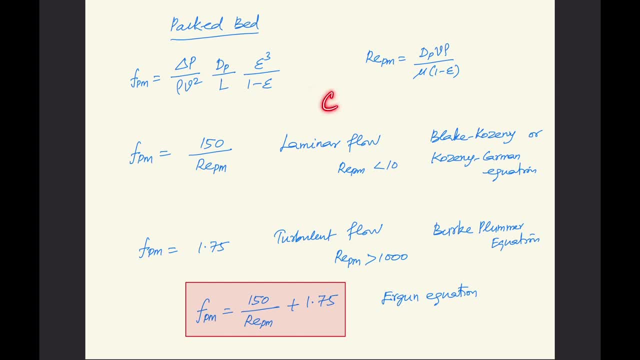 we know. we know this f is cd equal to 24 by rep. where in which we have re particle, this is re porous medium. otherwise the idea of connecting this is in the laminar flow. we have the same kind of dependency of f versus renal number. for turbulent region region this f is almost a constant say in the 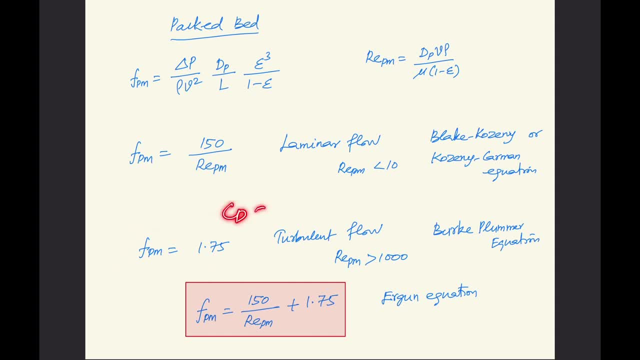 case of flow around a sphere, cd is taken as 0.44, and also in the case of flow through pipeline, even f is also almost a constant in this turbulent regime. so okay, this laminar part of this equation is valid for repm of less than 10, which is called as this block a questiony, or? 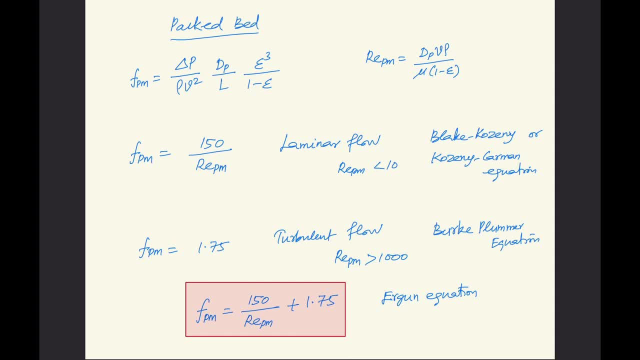 carmen equation: the highly for turbulent flow of our repm greater than 1000, we have this fpm equal to 1.75, which is also known. this equation is also known as parquet blummer equation. this total equation, that is, this laminar and turbulent point combined together, is called 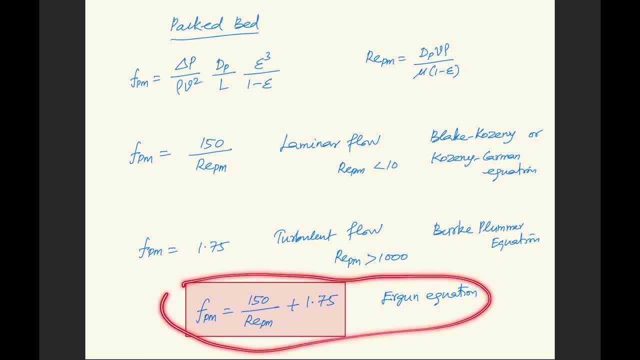 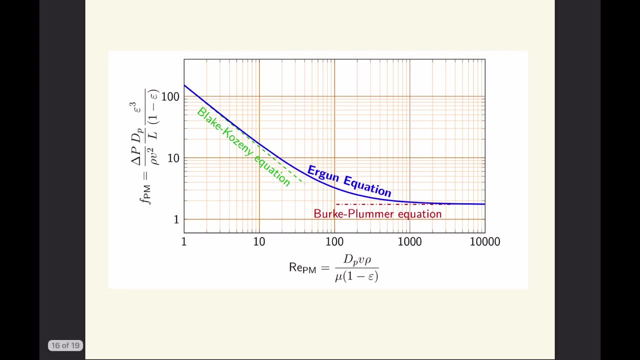 as the ergen equation. this is the most used equation in the packed bed and as well as in fluid aspect conditions. okay, this, uh, this is a plot of this block. a quotient per k plumber and ergen equation, what is called as fpm versus repm. as already said, fpm less than 10 laminar is valid. 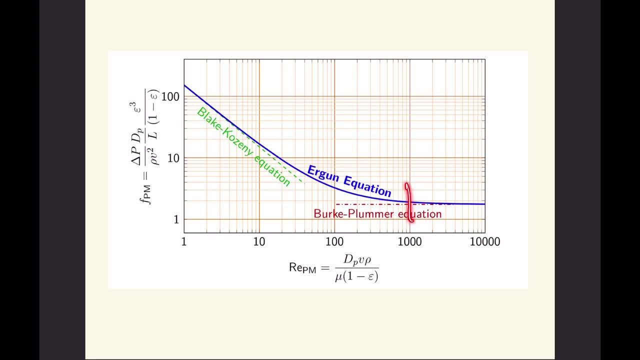 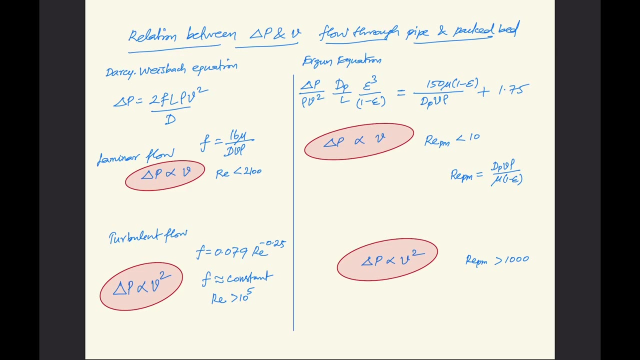 for repm greater than 1000, turbulent part is valid. otherwise use the generic equation, what is called as a ergen equation. this is about connecting this delta p and velocity for flow through p pipe and back to bed. so already we know this. delta p is equal to 2fl. rho v square by d. 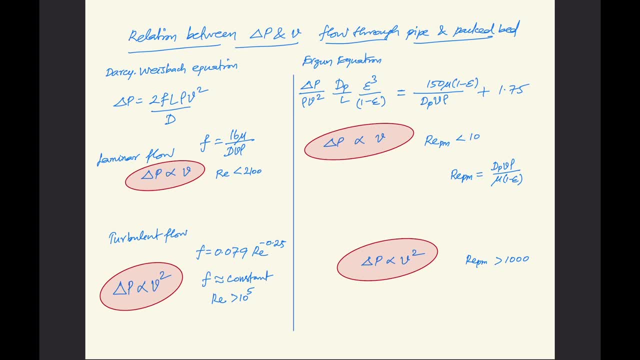 and from ergen equation we have this delta p. by rho v square. we have this if you check for laminar flow conditions. for laminar flow conditions f is equal to 16 by reynolds, number from which we have delta p is proportional to v. even from ergen equation also, we have the same dependency delta. 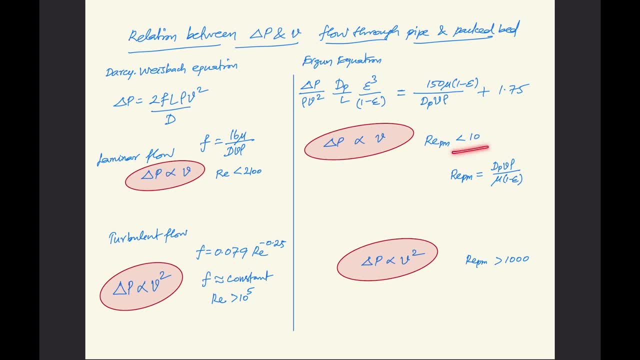 p is proportional to v. this is valid for less than repm, less than 10, whereas here we have re less than 2100. for turbulent flow, delta p is proportional to v square in the case of pipe flow, and here also we can easily say that delta p is. 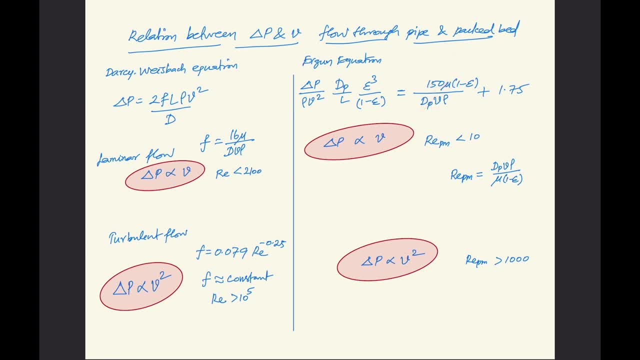 proportional to v square, otherwise this term will be zero. so delta p is proportional to v square in turbulent flow through packed but as well. so again to say you, using pipe flow equation itself, if you know the five flow equation, you can also say about the functional dependency for flow. 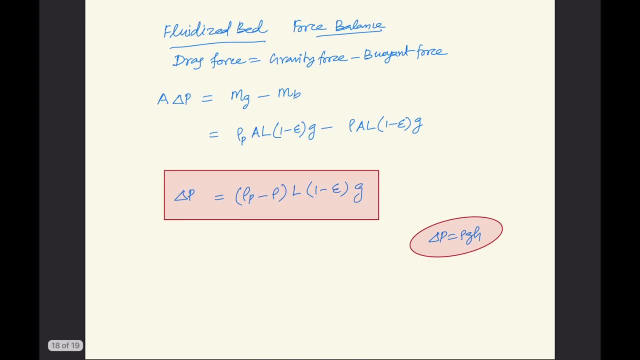 through packed. but okay, coming to this last equation, what is called as the fluidest bed conditions, the fluidest bit is formed, uh, at the. whenever there is, a balance is met with the drag force there is upward force is equal to the downward force, and this upward force is what is called the drag force, which is, uh pressure drop multiplied by the. 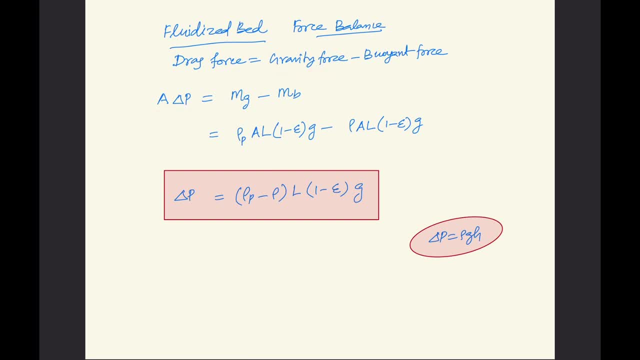 area and the gravitational force m in m, m into g, actually mg, mg, otherwise what is it? this is two be uh. you can write like uh, yeah, one minute. so this is to be uh. gravitational forces fg and this is bion forces, fb. so uh, this gravitational force is again volume into density, into, 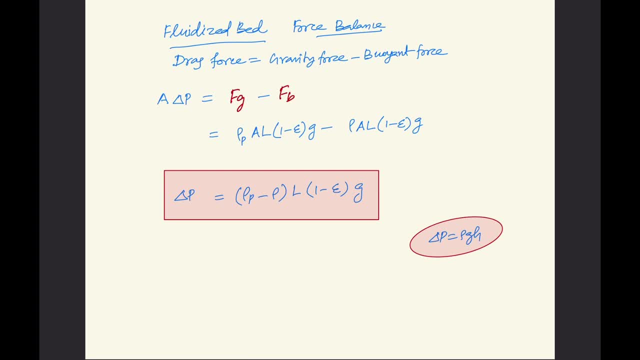 g, this volume to density will be getting. uh, what is it? uh, mass mass, into g, this acceleration. so so, this is, this is density, and this a, l into one minus e is the volume of the solid. uh, why do we have one minus e? because a and l refers to the total volume of packed bed and out of which you have to subtract this: 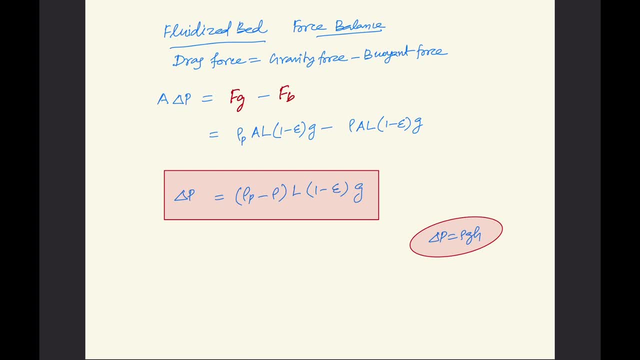 empty volume, which is one minus uh. otherwise, this uh one minus e refers to the volume of the solid. e is the volume of the uh voids. one minus is the volume of the solid, so the we have this volume of solid multiplied by density of solid. so this is the volume of the solid, so this is the volume of the. 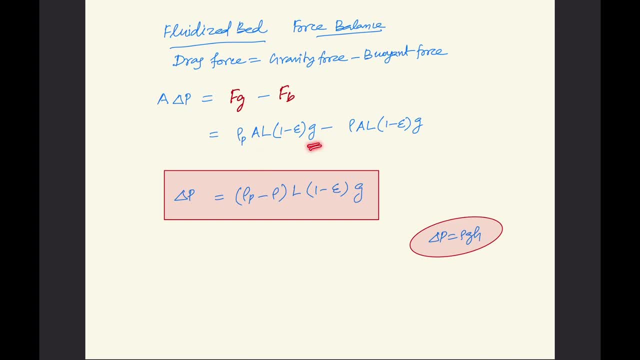 density of solid. so this is mass of solid multiplied by g. the same way, mass of fluid displaced is this quantity multiplied by g. okay, otherwise, if you cancel out this a on both sides, we have delta p equal to rho, p minus rho into l, into 1, minus epsilon into g, or is this also have? 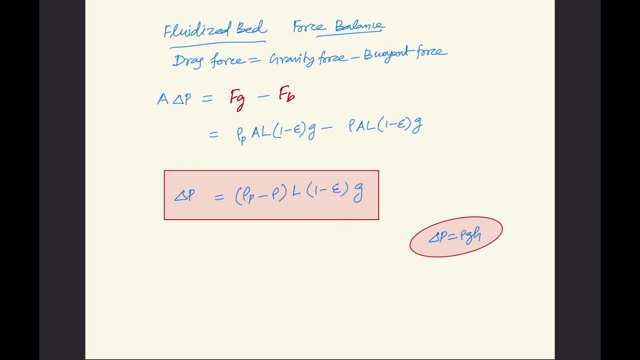 a functional dependency like delta, p is equal to rho, gh. in what way this is? you can take it as rho and this is g and this is h. of course, one minus epsilon is coming because to account for the fraction of solid which is only offering for the gravity and band forces. okay, this is a summary of equations. 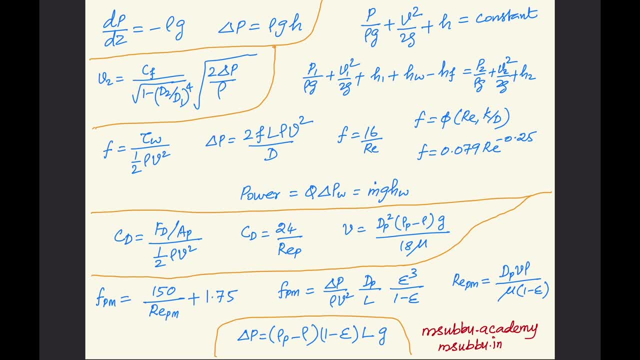 quickly see. we can see it again: everything db by d is that equal to minus rho g. otherwise, for incompressible fluid, delta p equal to rho gh and for manometric fluid the equality of pressure at the same level in a continuous connection of fluid and from vernal. 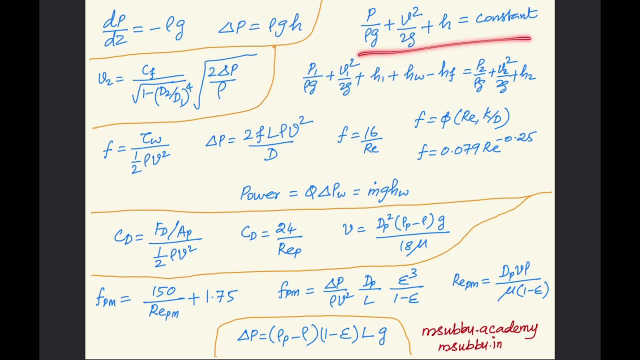 fluid flow, we have this bernoulli equation: p by rho g plus v, square by 2g plus h, equal to constant, including this head added by the pump and head loss due to friction, we have this equation and for flow meter, this bernoulli equation is reducing to this form: 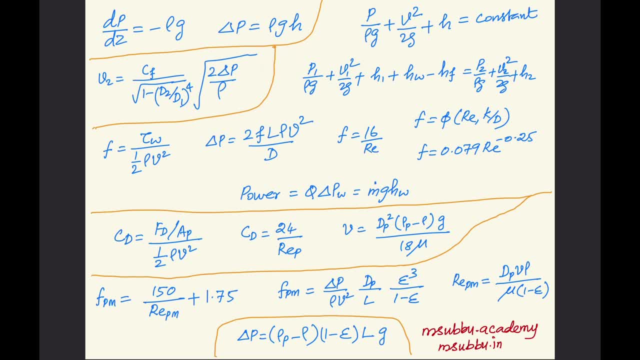 coming to this form. this term, this delta p, is a variable with what is called a venturian orifice meter, whereas this, this term, is a variable with rotameter. or is this delta b? delta b is remaining constant with rotameter, that delta b is nothing but the. 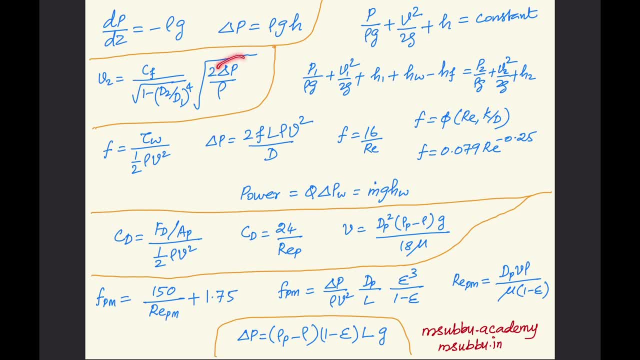 what is it? net downward force that is. this delta b is due to the drag force on the sphere, on the float, which is balanced by the net downwards force, which is gravity minus buoyancy. there is a constant. that's why this delta p is remaining constant with rotameter, whereas this is a variable, whereas in 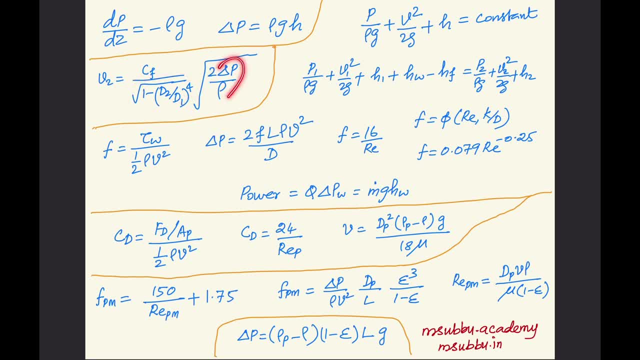 this case, the perfect form is a constant, which is v, so we have a constant will be given to this and this is a variable. okay, coming to the frictional thing, this: we have this definition of friction factor: f equal to tau, w by half, rho, v square, and from the equation we have this delta p. 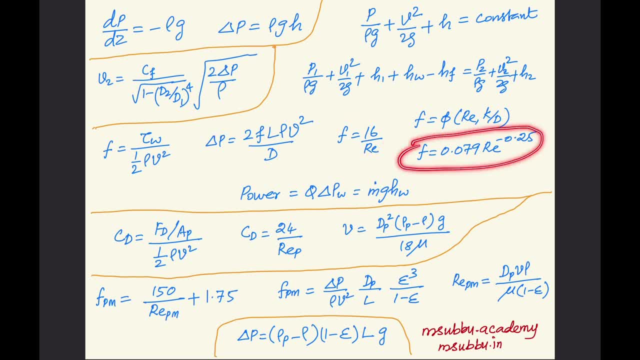 equal to 2. f, l rho v square by d, f equal to 16 by ranals number. otherwise, for laminar and f is equal the turbulent region. otherwise, f is a function of reynolds number and roughness factor. relative roughness k by d. and at last we need to interest, we are interested in getting the power required. 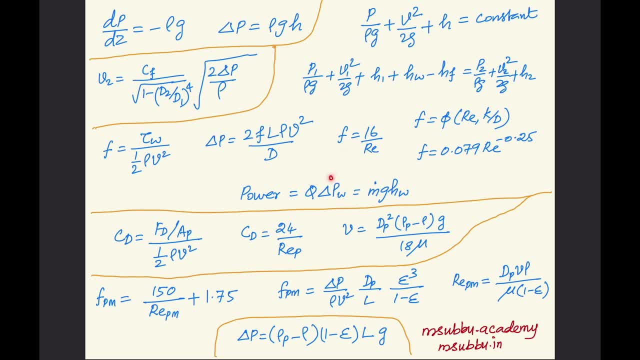 for pumping, which is q into delta, p across the pump, otherwise m dot, g into head ordered by the pump. okay, coming to the flow around solid, we have this definition of cd, what is called as the drag coefficient, which is fd by ap, by off row v square for reynolds number, less than 0.1. we have 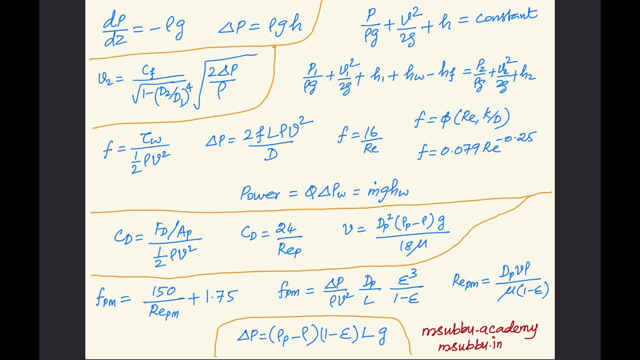 this creeping flow, for which cd equal to 24 by re particle. re particle is dp v rho by mu and from for the stokes law regime, or what is called for rep less than 0.1. we have this estimation of velocity, what is called as terminal settling velocity. we used to call that as which is given. 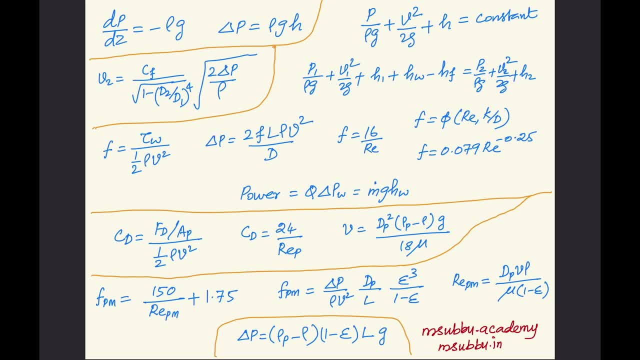 as dp square r, rho, p minus rho into g by 18 mu and for flow through bed of solid we have this fpm equal to 150 by repm plus 1.75. this is laminar part and turbulent part. laminar part is having this f. 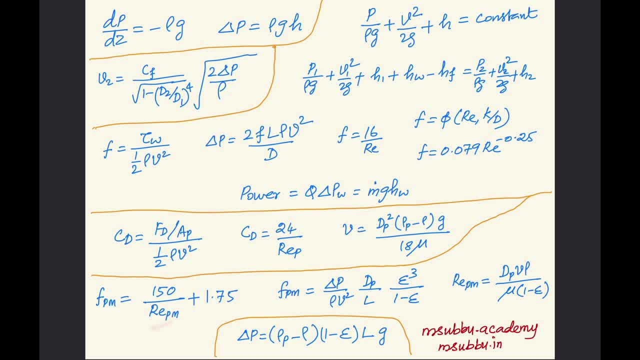 versus reynolds number, which is f is inversely proportional to reynolds number for turbulent part, f is nearly a constant. so fpm is given as delta p by rho v square into db, by l, into e cube by 1 minus e epsilon cube by 1 minus.